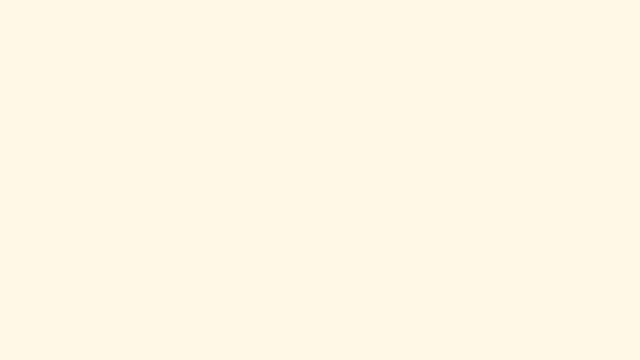 G'day, welcome to the TechMath channel. What we're going to be having a look at in this video is the easiest way to solve any question involving fractions, be they addition questions, subtraction questions, multiplication questions, or division questions. And we are going to go through and have a look at all of these. There's going to be a bit to go through, so please bear with us, but these are going to be the easiest way of solving any questions involving fractions. So we're going to start with addition questions. There's going to be about three types of questions you'll get with these. The first is where we have the same denominator, questions like this one here. Say, for instance, you are asking to add one-fifth plus two-fifths. Now, what you're going to notice straight away is that we have the same bottom number, the same denominator. If this is the case, what we do for our answer is we keep that same denominator. So in this case, the denominator is five. For our answer, the denominator will also be five. Now, for the numerator, the top number, all we do is add one-fifth plus two-fifths. So in this case, the denominator is five. 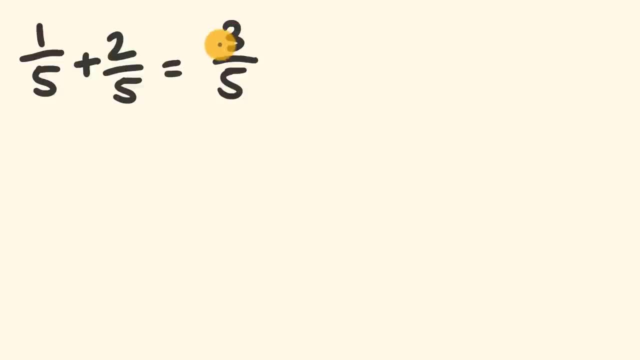 We just go through and add one plus two is equal to three. And that's how you add fractions with like denominators, with the same denominator. Keep that denominator in your answer and just add the numerators, add those top numbers together. But what about when we have different denominators? A question like this one here. Say we had one-quarter, and to this we wanted to add two-thirds. Now, the easiest way to do this is we're going to find a common denominator between the four and the three here. We have two different denominators, and we're going to find a common denominator. The easiest way to do that is through a bit of multiplication. First thing we do is we're going to multiply these denominators together. So four times three, that gives us the answer of 12. That gives us the denominator of our answer, which is 12. Now what we're going to do is starting at the top left here, we're going to multiply by the bottom right of these fractions here. So one multiplied by three. One multiplied by three is equal to three. What you're going to do is you're going to multiply by the bottom right of these fractions here. What you're going to notice is we've multiplied the four by three, and the three by three, so we've kept these fractions equivalent. Now what we're going to do is moving over to the right here, we're going to start with the top right number here, the two, and multiply it by 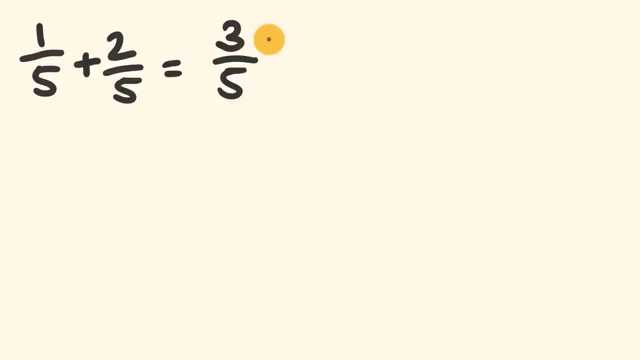 add the numerators, add those top numbers together. But what about when we have different denominators? A question like this one here: Say, we had one-quarter and to this we wanted to add two-thirds. Now the easiest way to do this is we're going to find a common denominator between. 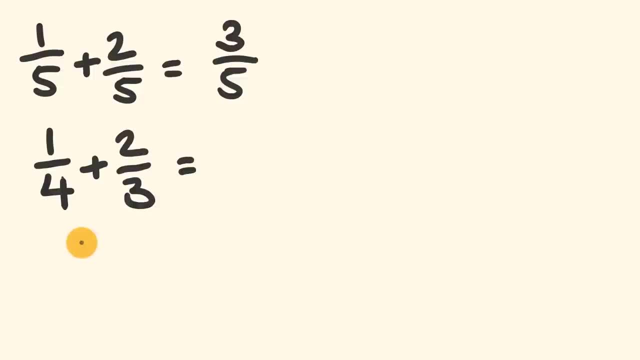 the four and the three. here We have two different denominators and we're going to find a common denominator. The easiest way to do that is through a bit of multiplication. First thing we do is we're going to multiply these denominators together, So four. 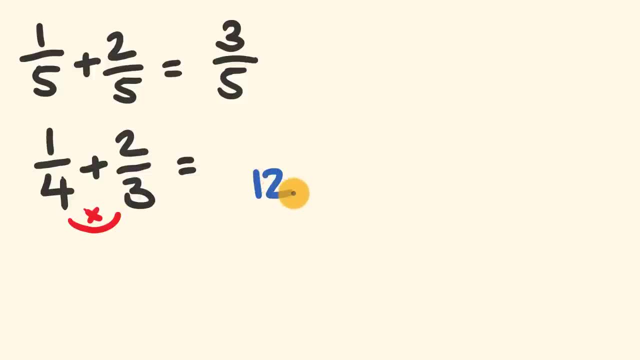 times three, that gives us the answer of 12.. That gives us the denominator of our answer, which is 12.. Now what we're going to do is, starting at the top left here, we're going to multiply by the bottom right of these fractions here. So one multiplied by three, One multiplied by three is: 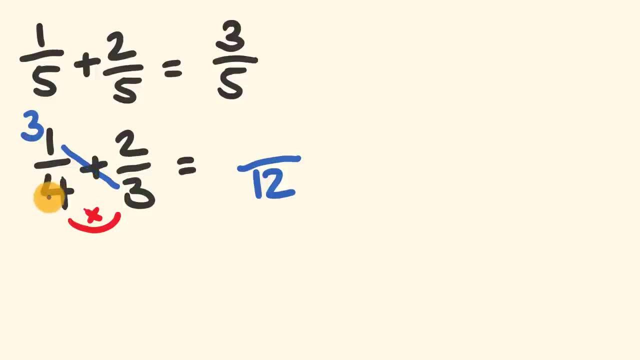 equal to three. What you're going to do is you're going to multiply by the bottom right of these fractions. here, What you're going to notice is we've multiplied the four by three and the three by three, so we've kept these fractions equivalent. Now what we're going to do is moving over to the. 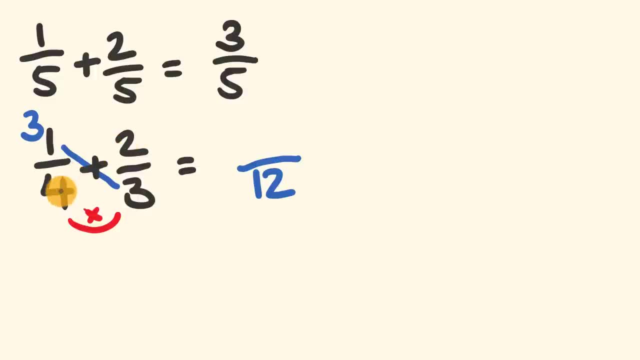 right. here we're going to start with the top right number, here, the two, and multiply it by the bottom left number. here Two multiplied by four is equal to eight. Once again, this just keeps the fractions equivalent We're adding. so we're just going to go three plus eight. This. 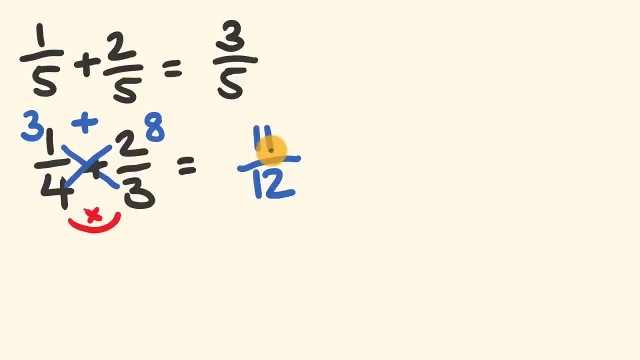 gives us our answer: 11 over 12.. Now that's a second type of question. what about? we have a look at a third type of question, and that's this one here, where we have mixed numbers, Something like one and a half plus four and two thirds- How we would go through and 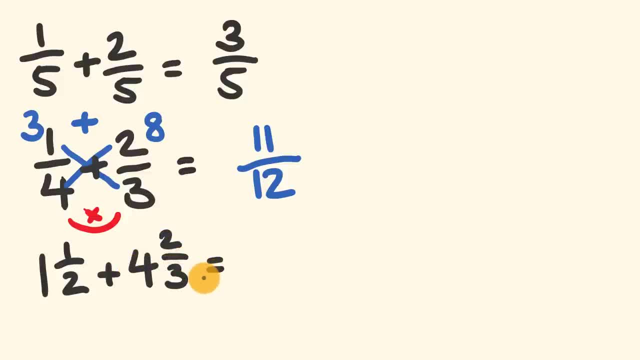 solve this Now. the way we do this is fairly simple. We're going to just turn these mixed numbers into improper fractions. That is just where they're simply fractions, but this is going to be a bigger number than the bottom number. You'll see what I mean. So let's do this The way. 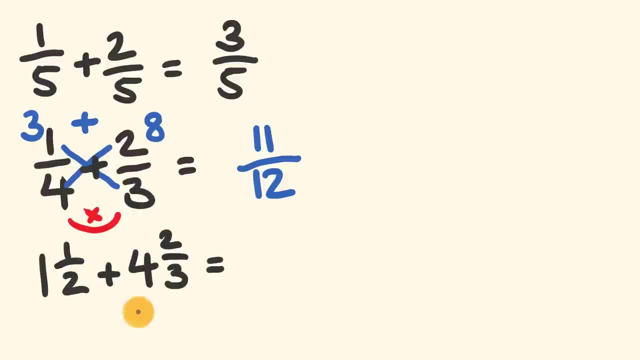 we do this is as follows: We're going to keep the same bottom numbers, the same denominators here, So we're going to have a two and then we're going to have a three and then we're going to have a three. All right, we're going to be adding still, but what's going to go on the top? 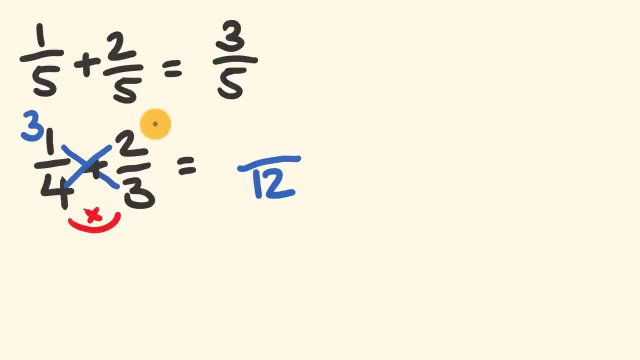 the bottom left number here. Two multiplied by four is equal to eight. Once again, this just keeps the fractions equivalent. We're adding, so we're just going to go three plus eight. This gives us our answer, 11 over 12. Now, that's a second type of question, 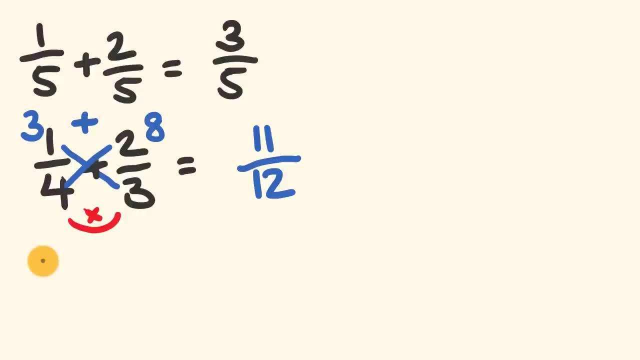 what about we have a look at a third type of question, and that's this one here where we have mixed numbers. Something like one and a half plus four and two thirds. How we would go through and solve this. Now the way we do this is fairly simple. We're going to just turn these mixed numbers into improper fractions. That is, just where they're simply fractions, but this is going to be a bigger number than the bottom number. You'll see what I mean. So let's do this. The way we do this is as follows. We're going to keep the same bottom numbers, the same denominators here. 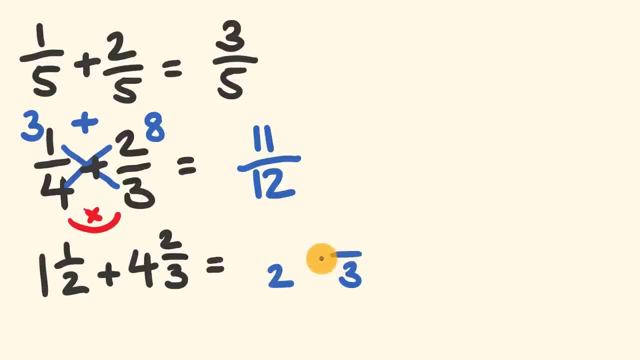 So we're going to have a two, and then we're going to have a three, and then we're going to have a three. All right, we're going to be adding still, but what's going to go on the top? 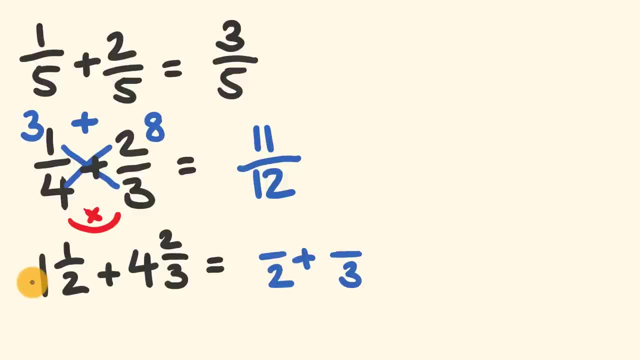 Well, we get this as follows. First off, we're going to multiply the whole number by the denominator. We have one times two, which is equal to two, and then we add that numerator. So one times two is two, plus one is equal to three. So we have three halves in one and a half. 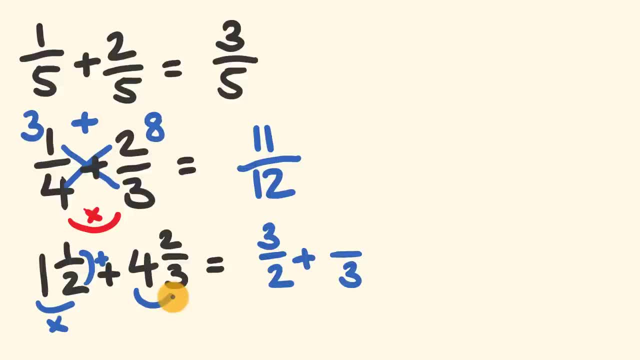 Now for four and two thirds, we do the same process. Four times three is equal to 12, 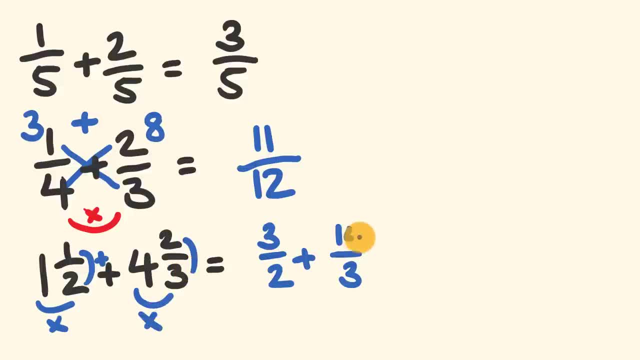 plus two is equal to 14. There you go. We have 14 thirds altogether. Now what we're going to do is we're simply going to go through and do the same process we did for this second fraction set 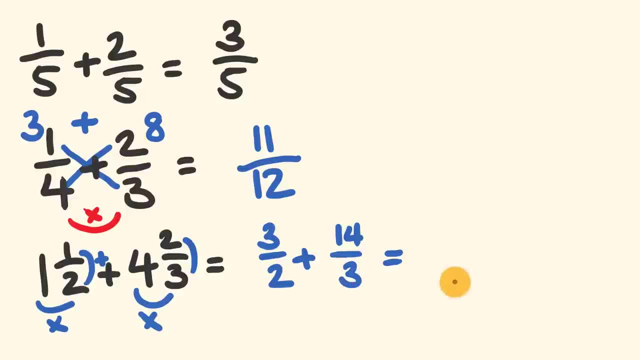 here. So let's do that. First off, we had two times three. This gives us the denominator. Two threes, a six. Now what we do is we're going to multiply three by three to give us nine, and we have 14 times two, which gives us 28. We're adding, so let's add those together. Nine, 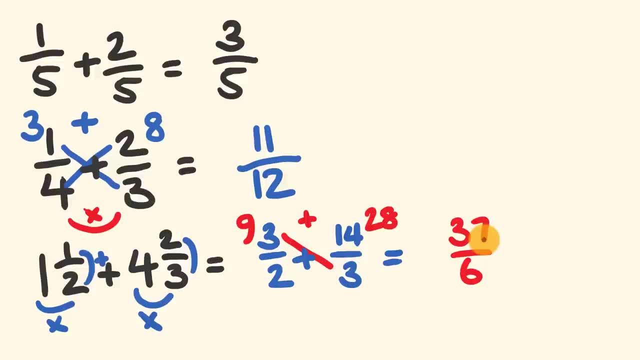 plus 28 gives us 37. So we have 37 sixths as our answer, but don't ever just leave this answer like this or your math teacher will be really annoyed at you. They're going to ask you to simplify this 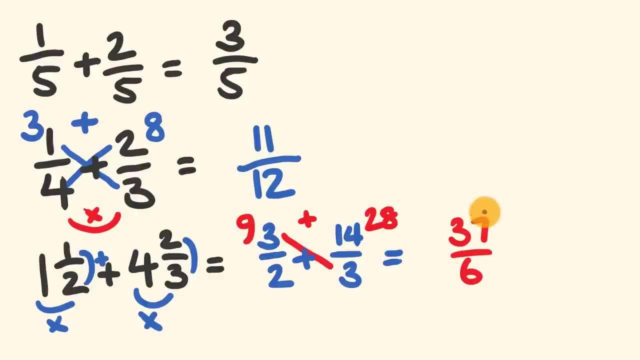 further. Now, how do we simplify this? Simple. This means 37 divided by six. Any fraction, even if it's this one here, means three divided by five, 11 divided by 12, and this one means 37 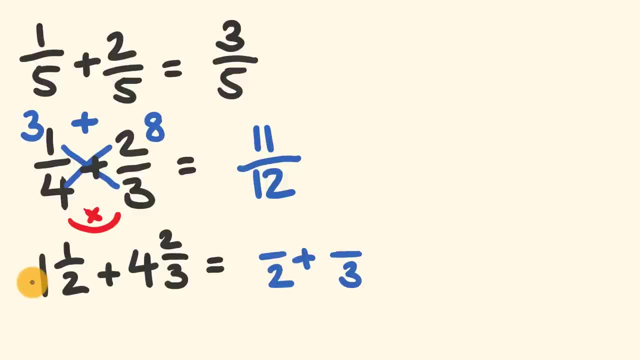 Well, we get this as follows: First off, we're going to multiply the whole number by the denominator. We have one times two, which is equal to two, and then we add that numerator. So one times two is two plus one is equal to three. So we have three halves in one and a half. 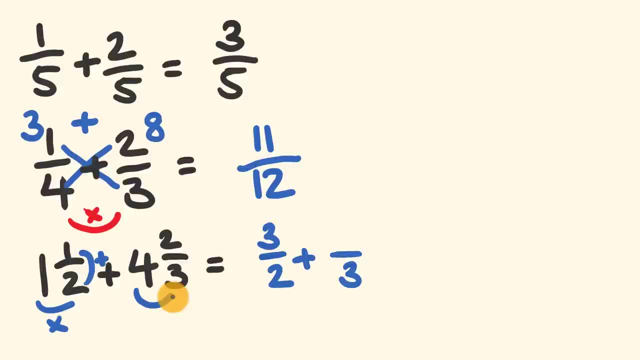 Now for four and two thirds. we do the same process. Four times three is equal to 12, plus two is equal to 14.. There you go, We have 14 thirds altogether. Now, what we're going to do is we're simply going to go through and do the same process we did for this second fraction set. 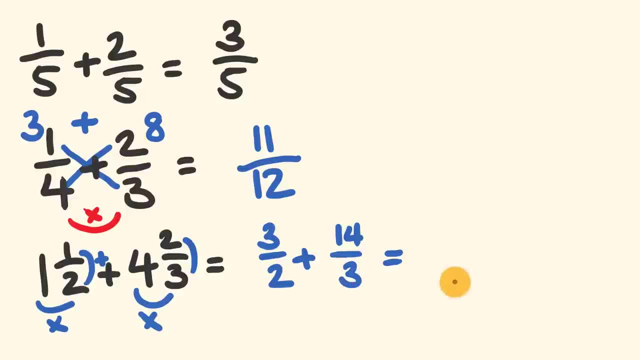 here. So let's do that. First off, we had two times three. This gives us the denominator Two, threes a six. Now what we do is we're going to multiply three by three to give us nine, and we have 14 times two, which gives us 28.. We're adding, so let's add those together: Nine. 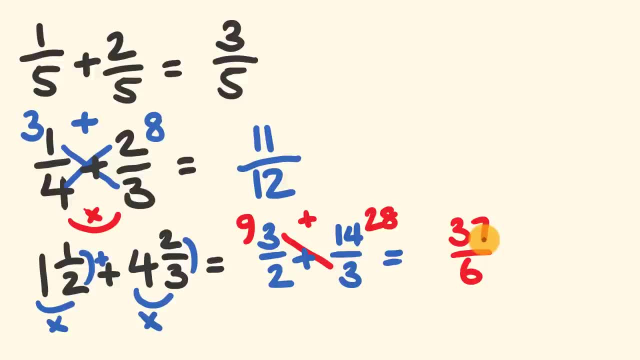 plus 28 gives us 37. So we have 37 sixths as our answer. but don't ever just leave this answer like this, or your math teacher will be really annoyed at you. They're going to ask you to simplify this further. Now, how do we simplify this Simple? This means 37 divided by six, Any fraction. 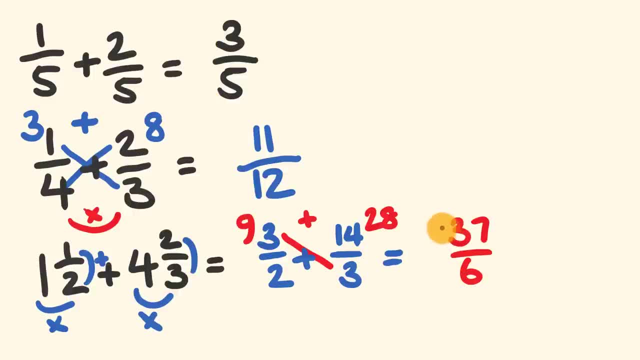 even if it's this one here means three divided by five, 11 divided by 12, and this one means 37 divided by six. So let's just do that: 37 divided by six. Well, six sixths is a 36,. 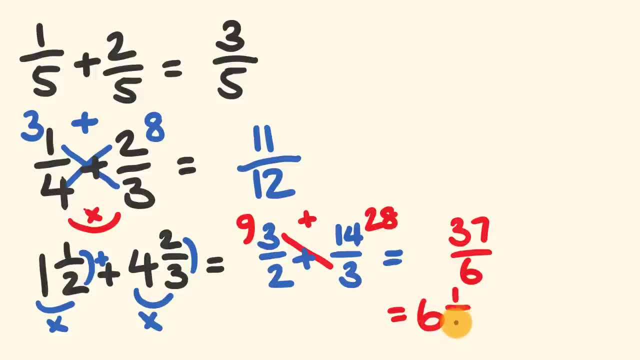 so the answer is going to be six and there is one left over. This one goes over that six at its same denominator. there, Cool, That's how you go through and you add any fraction together. Now you can probably guess how to subtract, because it's a very similar process. So let's. 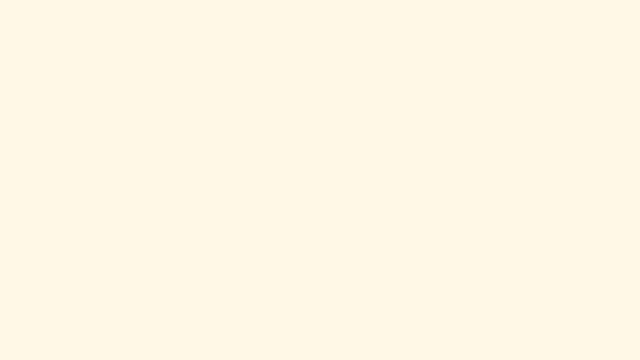 have a look. So when we're subtracting fractions, the process is very similar to addition. We're going to start off with a nice easy question. Say seven over eight minus one over eight. You should be able to get that one straight away. What do you think it is? 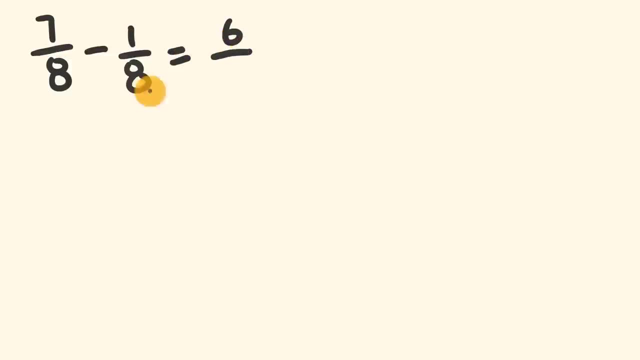 You've got it. Seven minus one is six, and that bottom number, the denominator, stays the same, It's six eighths. We can simplify this a bit further because we look for a number that goes into both the top and the bottom. Two goes into both the top and the bottom. 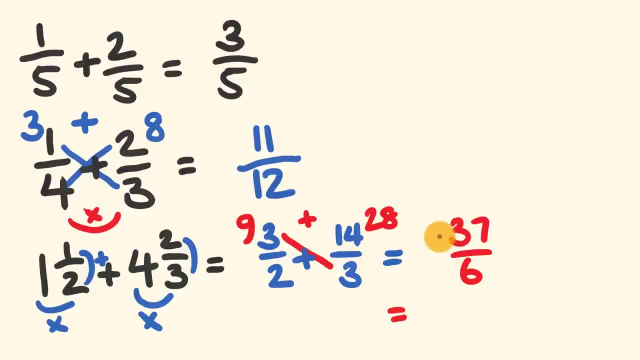 divided by six. So let's just do that, 37 divided by six. Well, six sixths is a 36, so the answer is going to be six, and there is one left over. This one goes over that six at its same denominator there. Cool. That's how you go through and you add any fraction together. 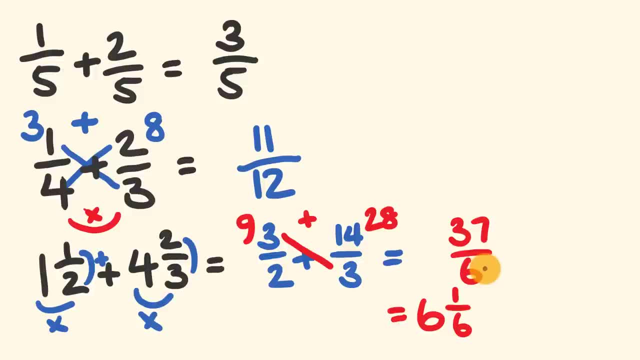 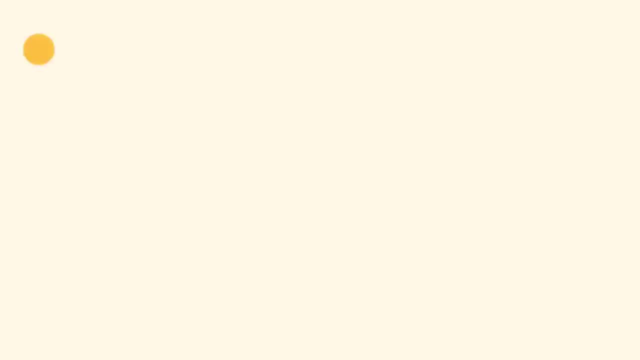 Now, you can probably guess how to subtract because it's a very similar process. So let's have a look. So when we're subtracting fractions, the process is very similar to addition. We're going to start off with a nice, easy question. Say seven over eight minus one over eight. You should be able to get that one straight away. What do you think it is? You've got it. Seven minus one is six, and that bottom number, the denominator, stays the same. It's six eighths. We can simplify this a bit further because we look for a number that goes into both the top and the bottom. Two goes into both the top and the bottom, 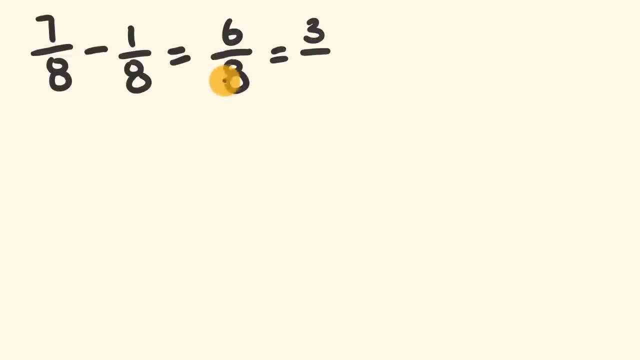 so six divided by two is equal to three, and eight divided by two is equal to four. 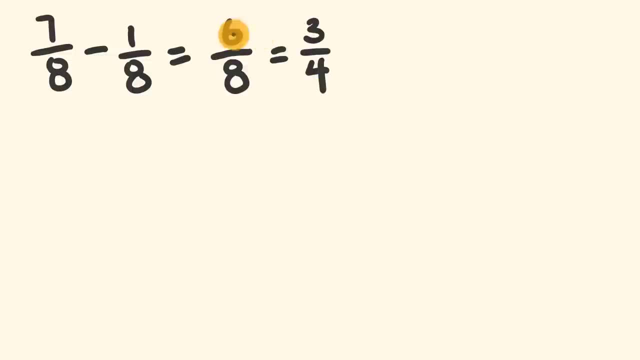 That's just a simplified version, equivalent version of six over eight. What about if we have a different denominator? Say we have something like this. Say we have four 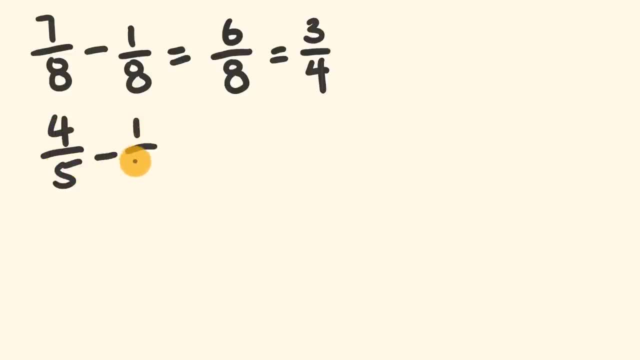 over five, and from this I want to subtract one third. Okay. I think you can guess how we're going to do this. To get the bottom number, we multiply. Five times three is equal to 15. Now, we do that cross multiplication, the cross working out four times three is equal to 12. One times five is equal to five. We are subtracting. Twelve subtract five. Our answer is seven. Really simple, right? Okay. 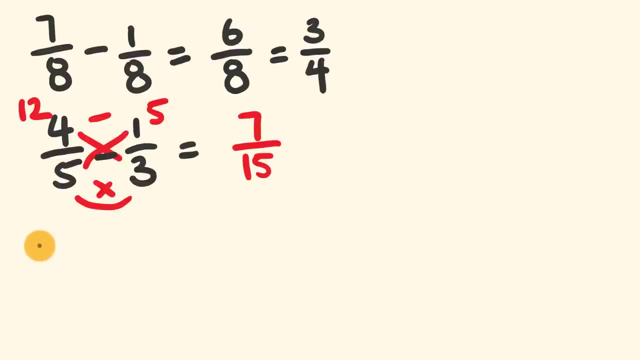 What about a mixed number here? So say we have something like, let's go three and one third, and from this I wish to subtract. Let's go two and a quarter, and see how this goes. 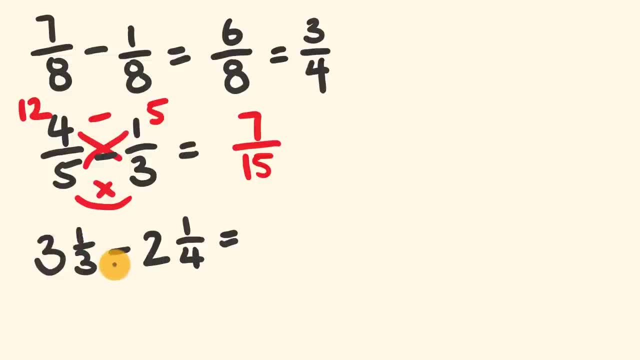 So with this, the first thing we're going to do is turn these mixed numbers into improper fractions, the same way as before. This is going to be a number over three, 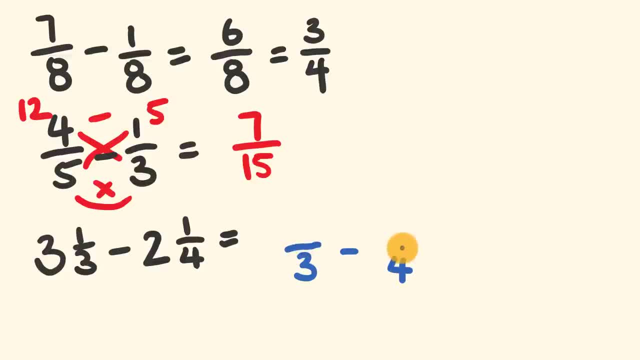 and this is going to be a number over four, and we are going to be subtracting. So let's do that. Three times three is nine, plus one is ten. 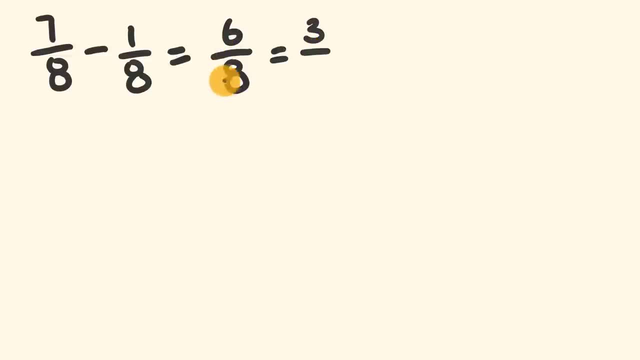 so six divided by two is equal to three and eight divided by two is equal to four. That's just a simplified version, equivalent version of six over eight. What about if we have a different denominator? Say we have something like this: Say we have four: 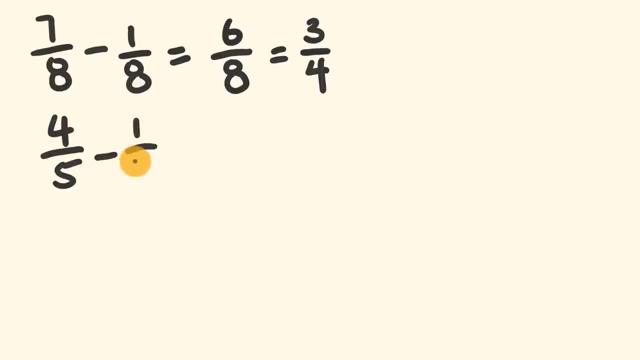 over five and from this I want to subtract one third. Okay, I think you can guess how we're going to do this To get the bottom number: we multiply Five times three is equal to 15.. Now we do that cross multiplication. the cross working out four times three is equal to 12.. One 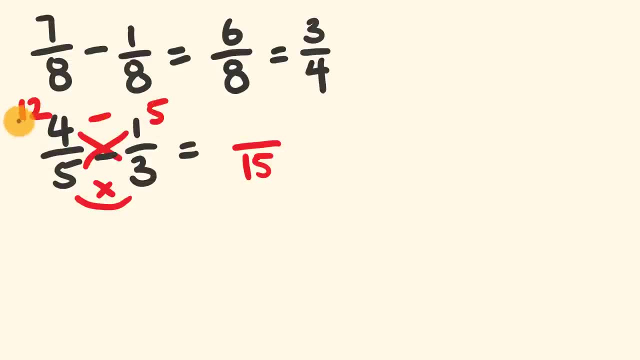 times five is equal to five. We are subtracting Twelve, subtract five, Our answer is seven. Really simple, right? Okay, What about a mixed number here? So say, we have something like: let's go three and one third, and from this I wish to subtract. Let's go two and a quarter and see how this goes. 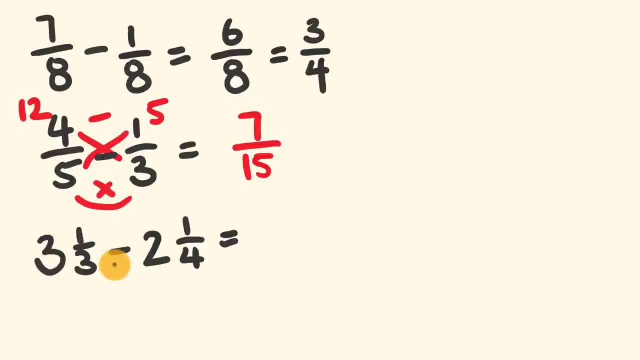 So, with this, the first thing we're going to do is turn these mixed numbers into improper fractions, the same way as before: This is going to be a number over three, and this is going to be a number over four, and we are going to be subtracting. So let's do that. 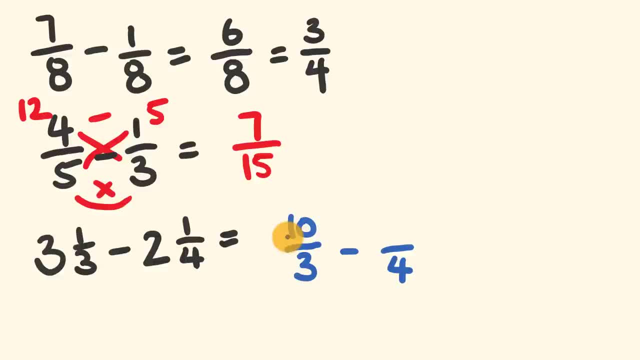 Three times three is nine plus one is ten. Two times four is eight plus one is nine. Now, what we're going to do is that same cross fraction-y sort of thing that we did over here. Okay, So let's do that. 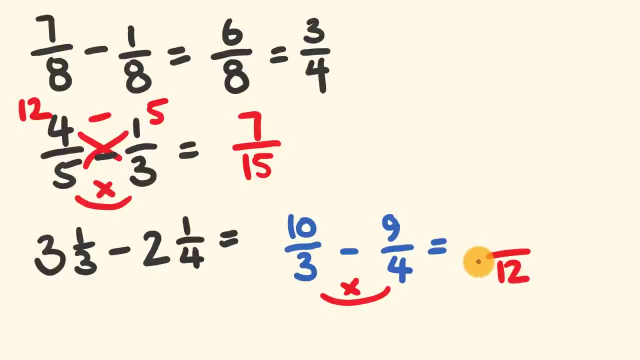 Three times four is equal to 12, and now we're going to do this bit of working out: Ten times four is equal to 40.. Three times nine is equal to 27.. We're subtracting Forty. take away 27 is equal to 13.. All right, Can we leave it like that? 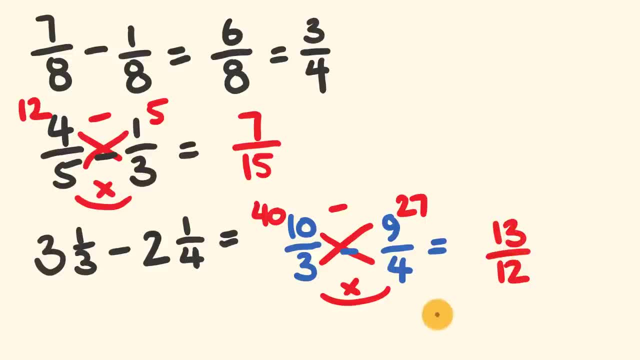 You've got it. This is an improper fraction. We're going to have to change it, So let's do that. 13 divided by 12 is equal to one, and there's one left over. That's 1 over 12.. 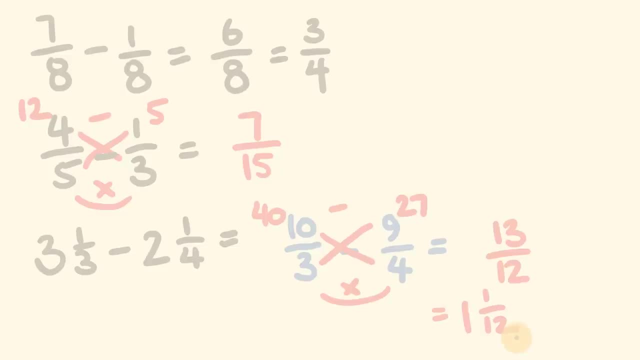 Cool. Now let's have a look at multiplying fractions. All right, So multiplying fractions is nice and easy. I think it's the easiest operation you can do with fractions. I remember as a kid my brother told me this and it's always stuck with me and always helped me when I was. 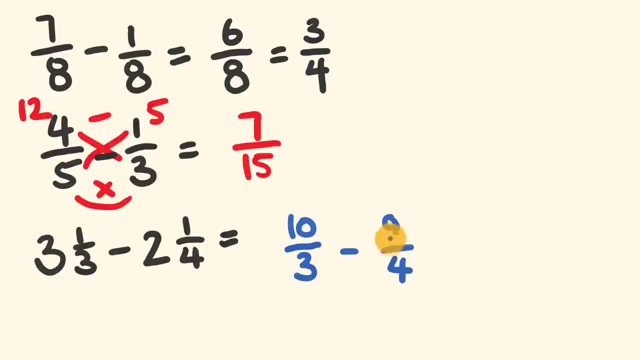 Two times four is eight, plus one is nine. Now, what we're going to do is that same cross fraction-y sort of thing that we did over here. Okay. So let's do that. 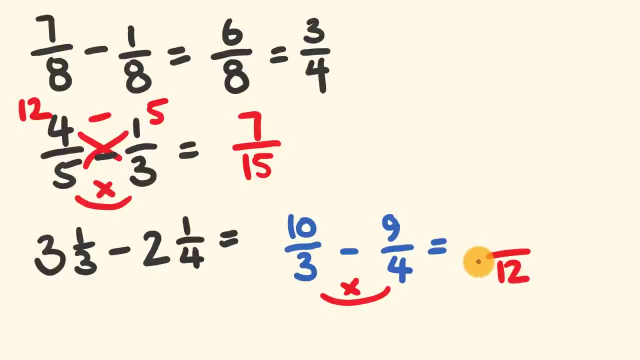 Three times four is equal to 12, and now we're going to do this bit of working out. Ten times four is equal to 40. Three times nine is equal to 27. We're subtracting. Forty take away 27 is equal to 13. All right. Can we leave it like that? 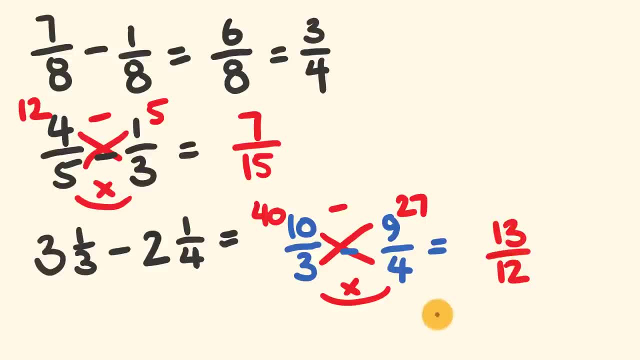 You've got it. This is an improper fraction. We're going to have to change it, so let's do that. 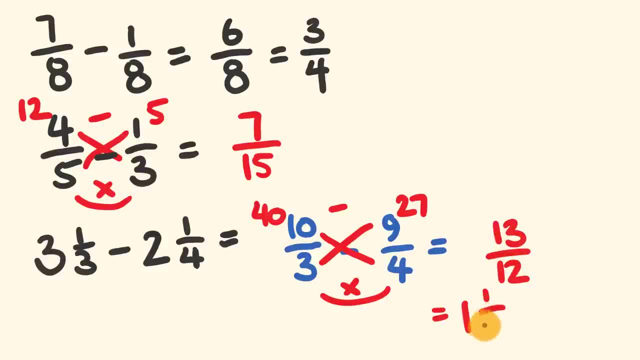 Thirteen divided by 12 is equal to one, and there's one left over. That's one over 12. 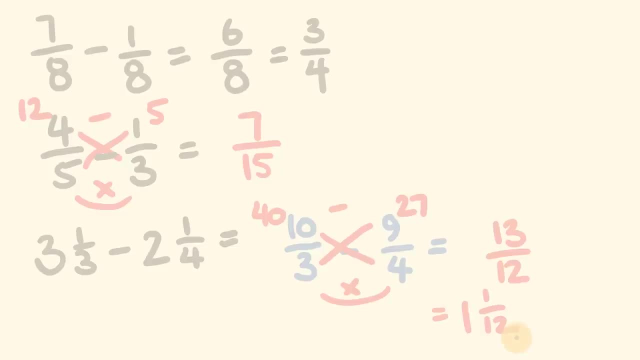 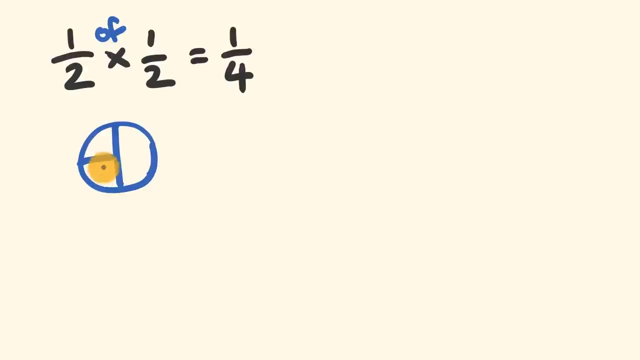 Cool. Now, let's have a look at multiplying fractions. All right. So multiplying fractions is nice and easy. I think it's the easiest operation you can do with fractions. I remember as a kid, my brother told me this, and it's always stuck with me, and it always helped me when I was trying to remember how to multiply fractions. He remember he told me when I was very little, I wasn't in school yet, a half multiplied by a half is equal to one quarter now that was a little bit strange you know how did you multiply by something and get a smaller number all right nobody value aside it did help me to remember this and it makes perfect sense because what's a one half of a half another way of thinking of this a half of a half well if you think of that with a pizza for instance or a pie you cut that in half you have half a pizza and then half of that is one quarter of a pizza right all up we have one quarter a half of a half is equal to a quarter all right so the way that we do this uh it's not just to remember my little childhood stories just have a look at this one multiplied by one is equal to one two multiplied by two is equal to four top by the top bottom by the bottom got your answer happy days so let me give you a harder question here so say for instance 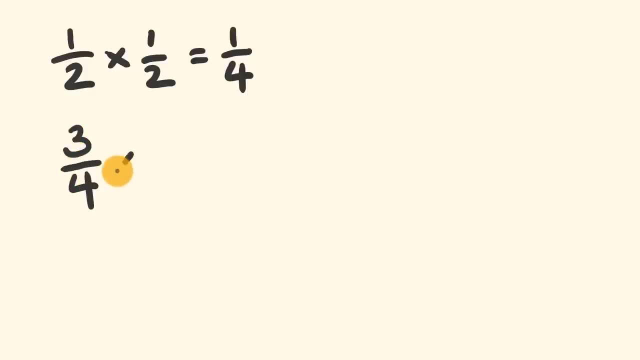 we wanted to go what's three quarters multiplied by one 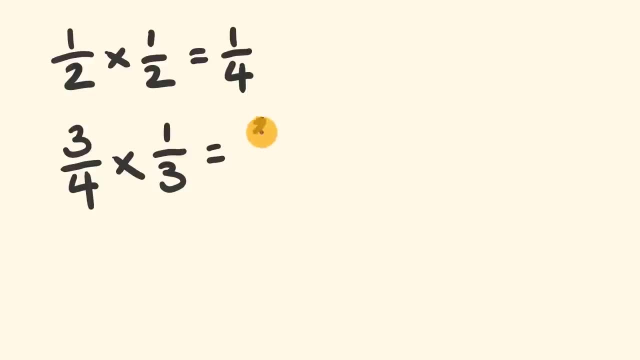 third okay nice and simple three times one is equal to three four times three is equal to twelve 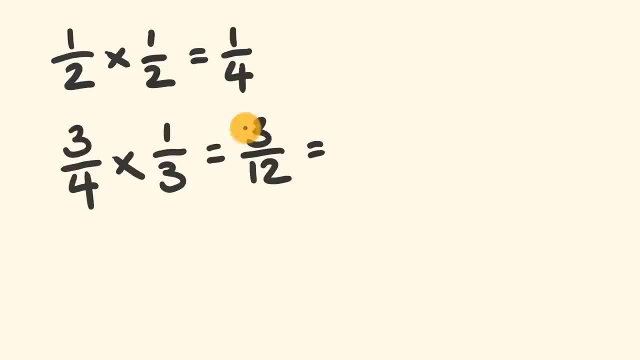 uh now that's our answer but we can simplify this further into equivalent fractions you know a bit smaller because there's a three that goes into both the top and the bottom divide by three 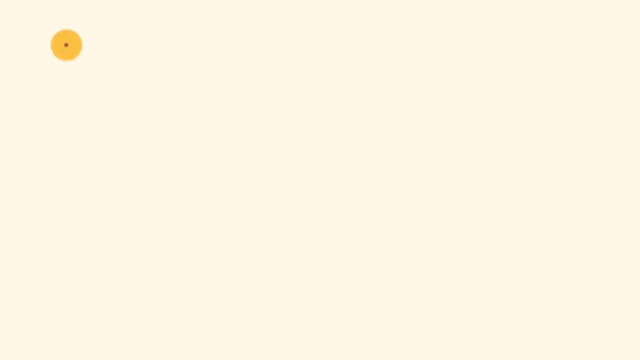 trying to remember how to multiply fractions, He told me when I was very little- I wasn't at school yet- that a half multiplied by a half is equal to one quarter. That was a little bit strange. You know how did you multiply by something and get a smaller number? All right, Knowledge value. 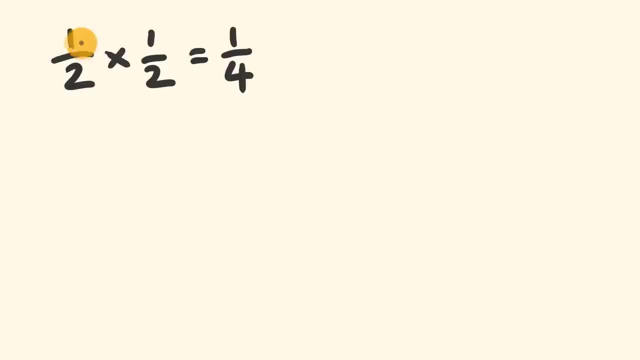 aside. it did help me to remember this and it makes perfect sense, because what's a one, half of a half? Another way of thinking of this: A half of a half? well, if you think of that with a pizza, for instance, or a pie, you cut that in half. you have half a pizza and then half of. 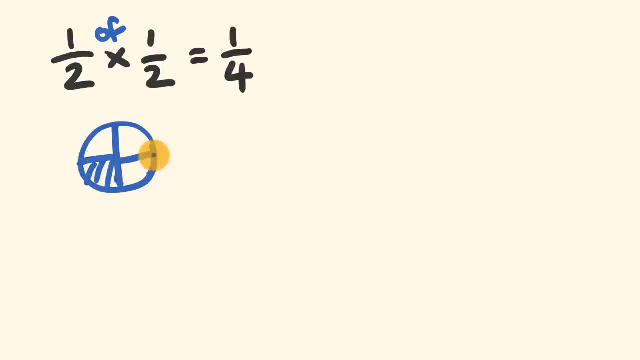 that is one quarter of a pizza right. All right, We have one quarter. A half of a half is equal to a quarter, All right. So the way that we do this is not just to remember my little childhood stories. Just have a look at this. One multiplied by one is equal to. 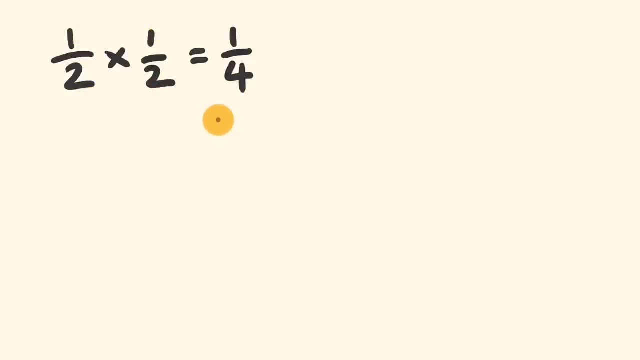 one Two multiplied by two is equal to four. Top by the top, bottom by the bottom. Got your answer, Happy days. So let me give you a harder question here. So say, for instance: we wanted to go: what's three quarters multiplied by one? third? Okay, 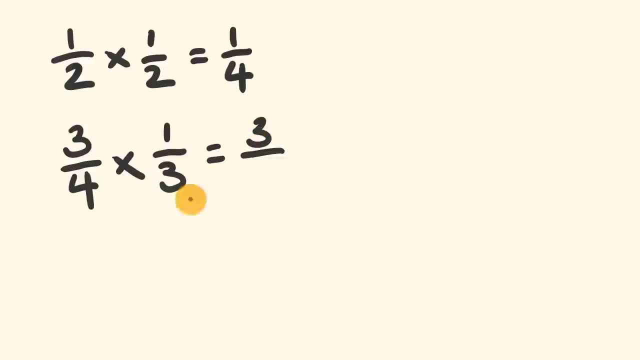 Nice and simple. Three times one is equal to three. Four times three is equal to 12.. Now that's our answer, but we can simplify this further into equivalent fractions, you know a bit smaller, because there's a three that goes into both the top and the bottom. 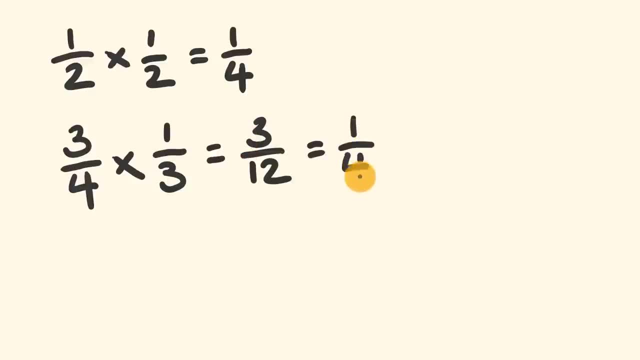 Divide by three, divide by three, we get one over four. Our answer is one quarter. Cool. Now just one last thing. What do we do if we have a whole number? Well, if we have a mixed number before we do the same like we did before. 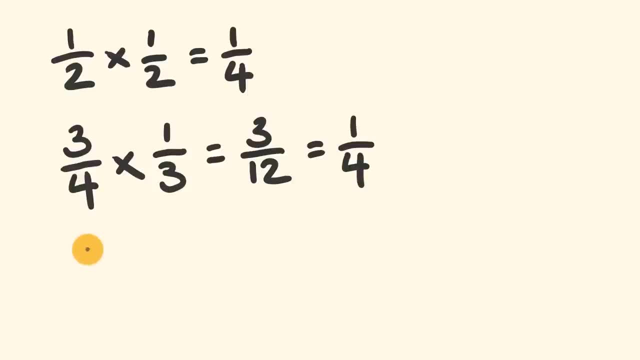 There's nothing major there, but in particular, I want to show you something like this. Say, for instance: I wanted to know what half multiplied by seven was. Now, the easiest way to deal with this is as follows: We're going to keep that half the same and we're multiplying. 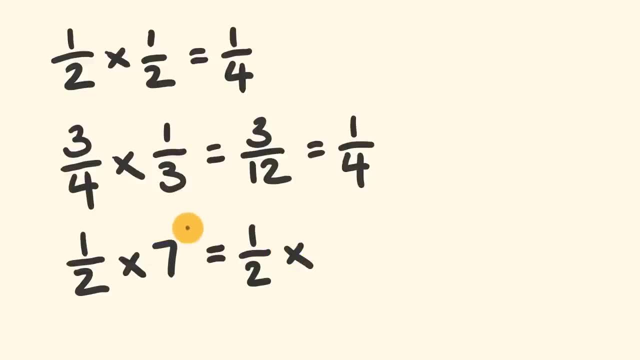 by this seven, which we're going to turn into a fraction. Now, this as a fraction is equal to seven over one. All right, Makes sense, because seven divided by one is equal to seven. All right, This is seven as a fraction. Now we can go through and solve this really easy, right. 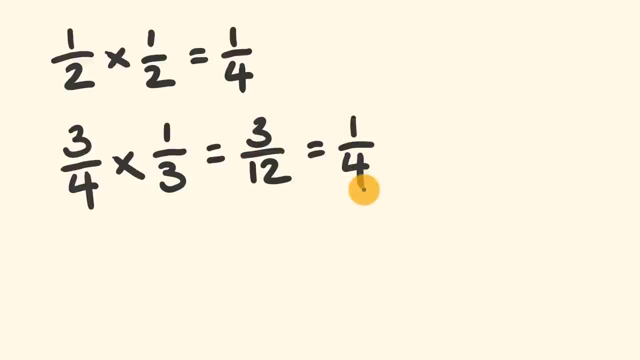 divide by three we get one over four our answer is one quarter cool now just one last thing what 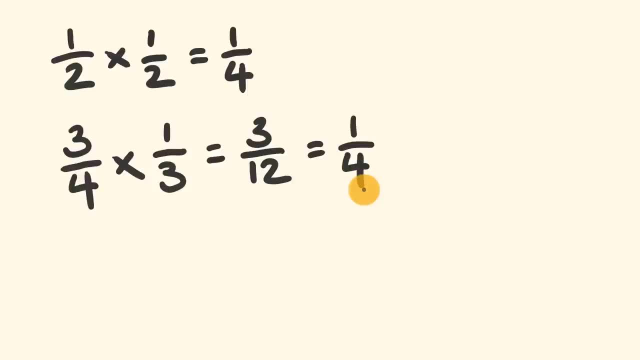 do we do if we have a whole number well if we have a mixed number before we 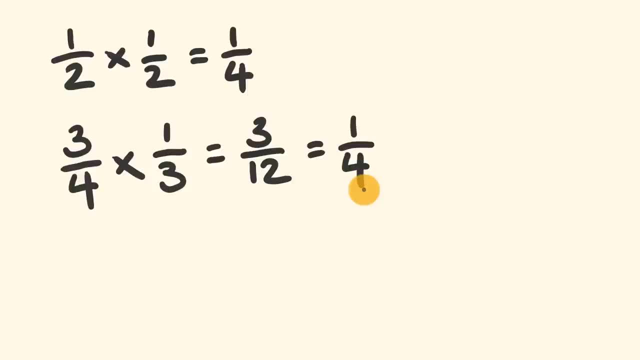 we do the same like we did before there's nothing major there but in particular i want to 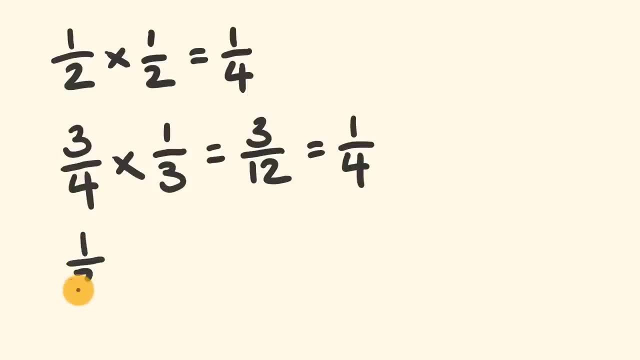 show you something like this so for instance i wanted to know what half multiplied by seven was now the easiest way to deal with this is as follows we're going to keep that half the same 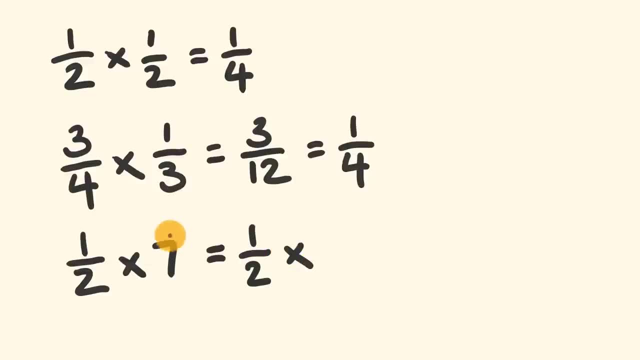 and we're multiplying by this 7 which we're going to turn into a fraction now this as a fraction is 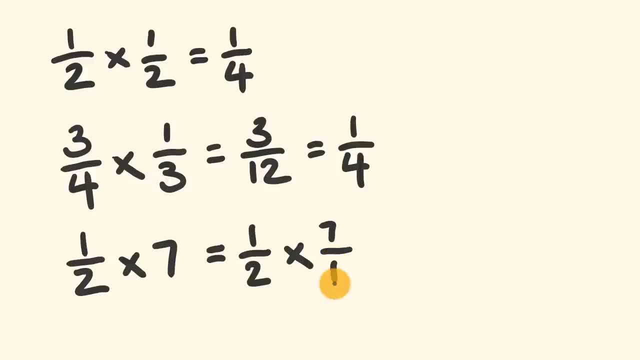 equal to 7 over 1. all right makes sense because 7 divided by 1 is equal to 7. all right this is 7 as a fraction. Now we can go through and solve this really easy right? 1 times 7 is 7. 2 times 1 is equal to 2. We can simplify this 7 divided by 2 is equal to 3 and there's 1 left over that's 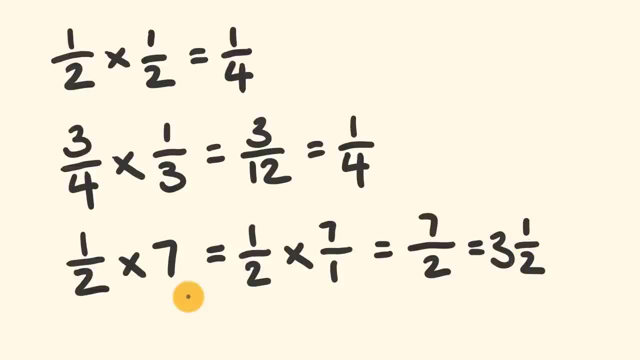 three and a half. What's half of 7? Well of course it's three and a half right? All right so now 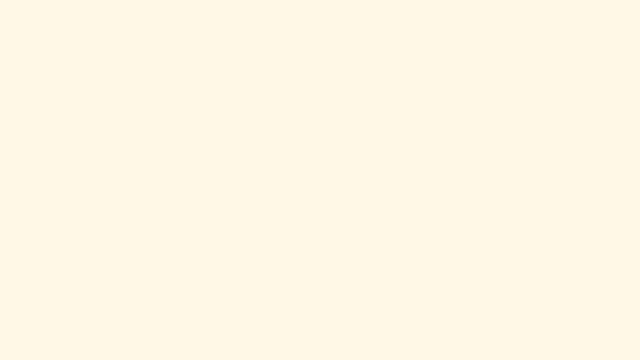 let's go have a look at division. So now we're going to have a look at dividing fractions and these are really easy to do as long as you remember the division is the opposite of multiplication. Now multiplication was pretty easy so there's just one extra step we need to do to turn it into the opposite. So let's do that. First off let's get a question up here. We have something like this one here three quarters and I want to divide into this one half. I want to see how many halves are in three quarters. All right so as I said the opposite of division is multiplication. So we're going to divide into this one half. So we're going to divide into this one half. We're going to rewrite this out a little bit. Three quarters and we're going to be multiplying. We're not going to be multiplying by a half. We're going to be multiplying by the opposite of a half. Now the opposite of a half well if you get this whole fraction here and you flip it on its head if you flip these around you get the opposite of one half. You have two over one. Okay now we've just turned it into a nice easy multiplication. So let's do that. Three times two is equal to six. Four times one is equal to four. We have six over four. We have six over four. 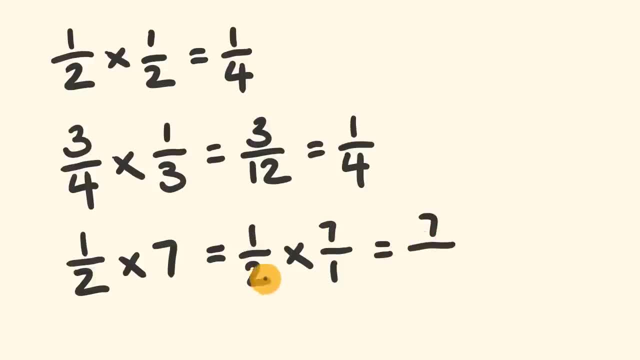 One times seven is seven. Two times one is equal to two. We can simplify this: Seven divided by two is equal to three, and there's one left over. That's three and a half. What's half of seven? Well, of course it's three and a half, right, All right. So now let's go have a look at division. 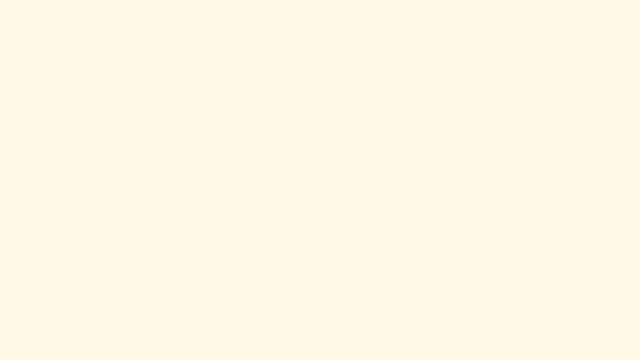 So now we're going to have a look at dividing fractions, and these are really easy to do, as long as you remember that division is the opposite of multiplication. Now, multiplication is pretty easy, So there's just one extra step we need to do to turn it into the opposite. 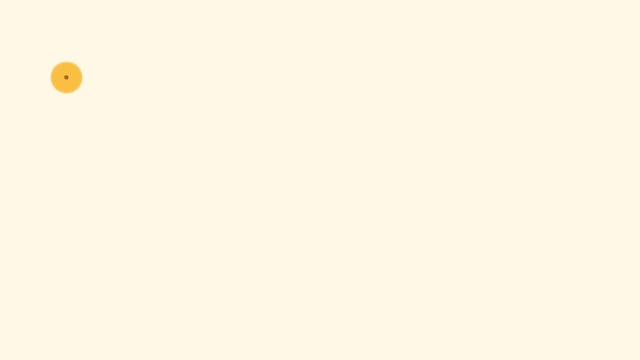 So let's do that. First off, let's get a question up here. We have something like this one here, three quarters, and I want to divide into this one half. I want to see how many halves are in three quarters, All right, So, as I said, the opposite of division is multiplication. So 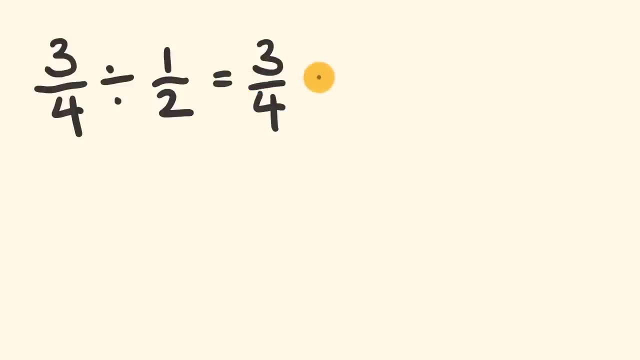 we're going to rewrite this out a little bit: Three quarters, and we're going to be multiplying. We're not going to be multiplying by a half, We're going to be multiplying by the opposite of a half. Now, the opposite of a half. well, if you get this whole fraction here and you flip it on its head, 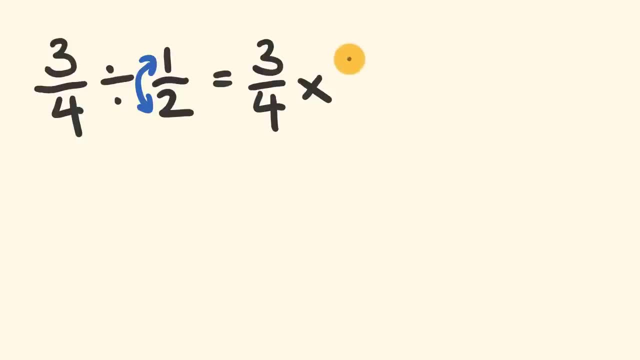 if you flip these around, you get the opposite of one half. You have two over one. Okay, Now we've just turned it into a nice easy multiplication, So let's do that. Three times two is equal to six. Four times one is equal to four. We have six over four. 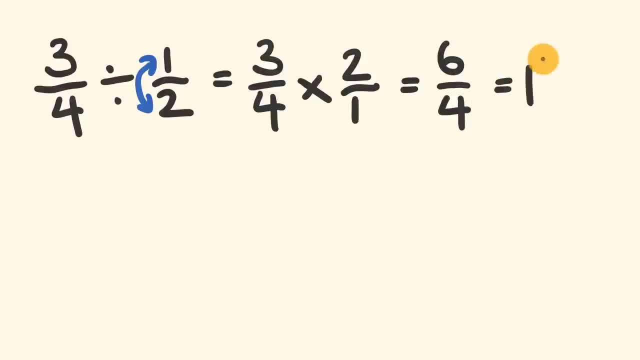 which is equal to, that's one and two left over two, four, And we can simplify this further Because two goes into both the top and the bottom. This is equal to one and a half Simple. right Now, what do we do if we have a whole number here? Well, no surprise here, Say I wanted. 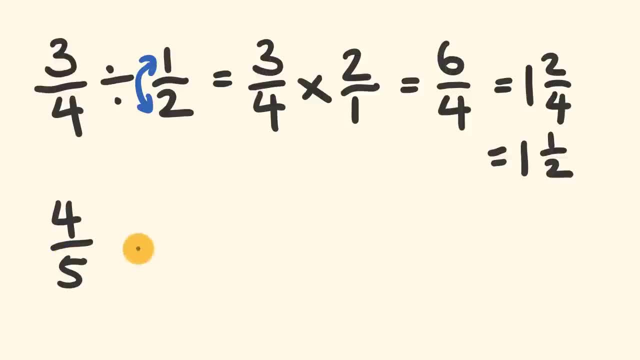 to go. what is four fifths, And I want to divide that by six. Okay, What would that equal? We're just going to do that same process here. We have four fifths and this is divided by six over one. 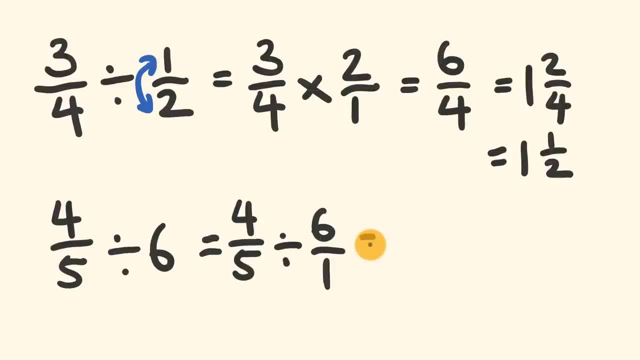 Now, we don't want to be dividing, We want to do a bit of multiplication here. So let's just change this around. We have four fifths And we're going to multiply by one over six, So let's do that. Now what we have is four times.